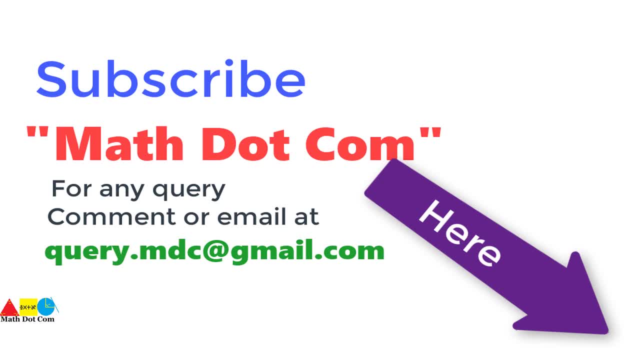 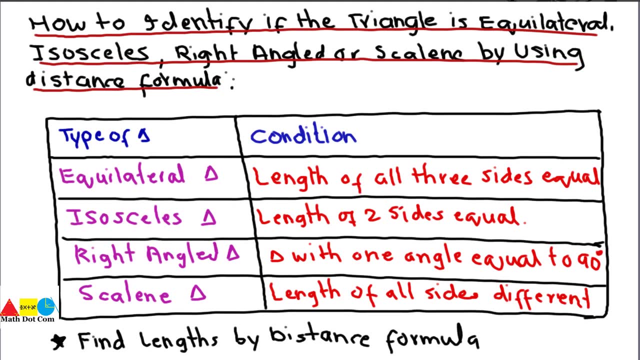 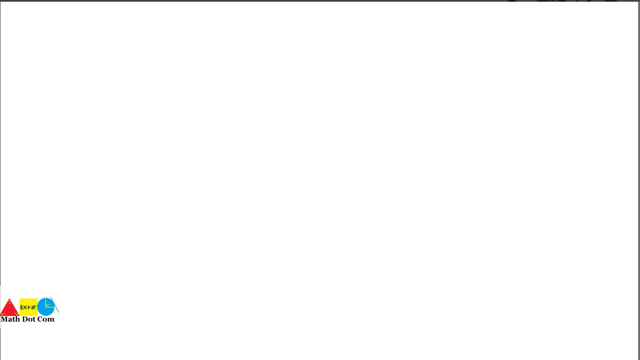 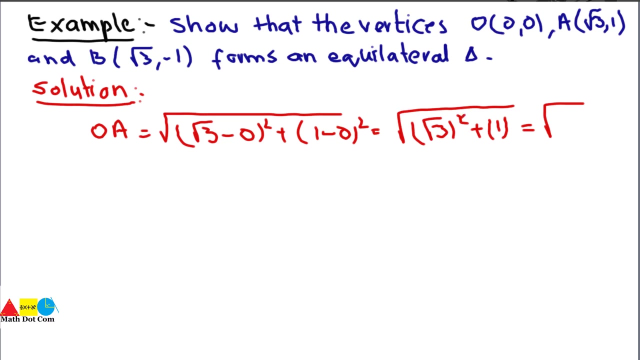 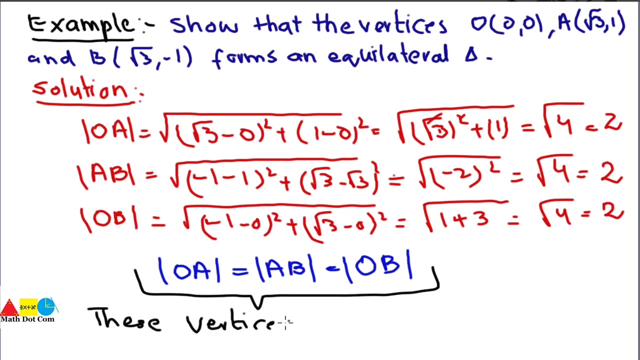 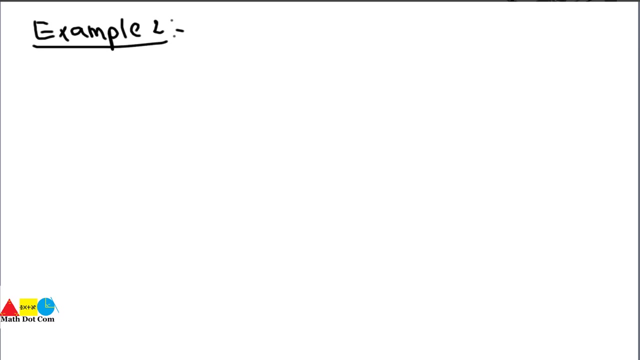 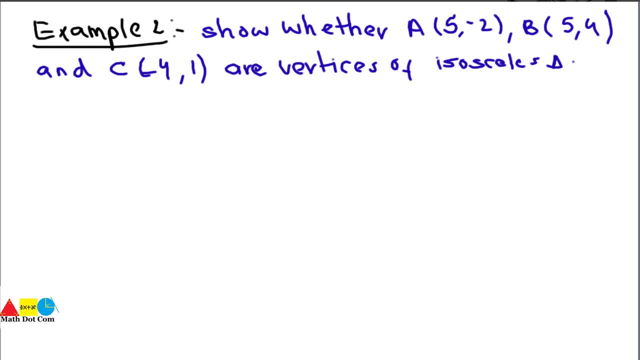 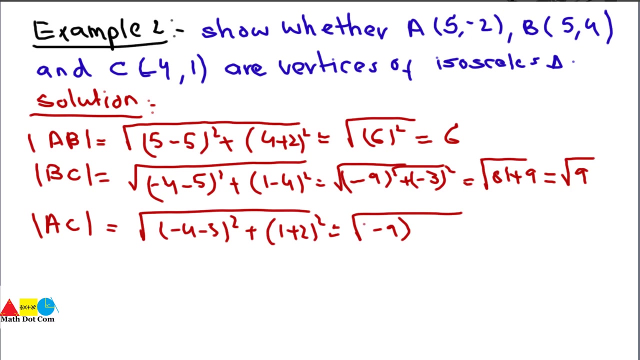 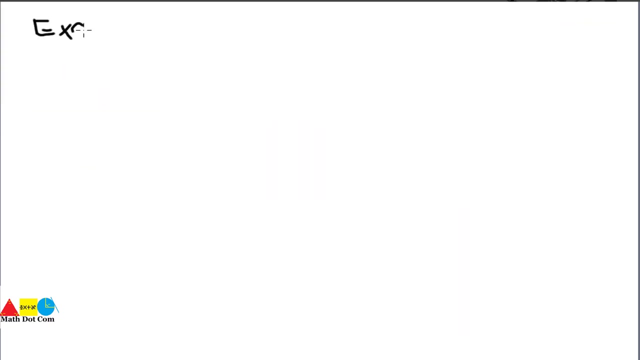 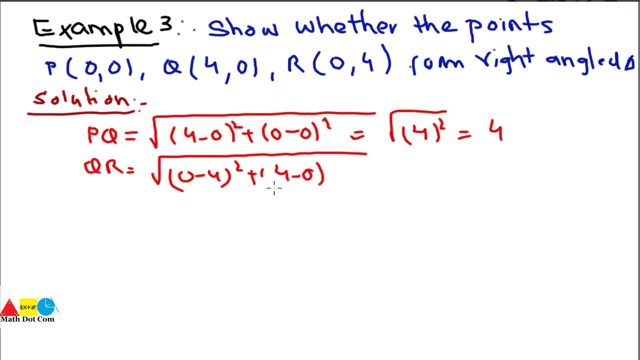 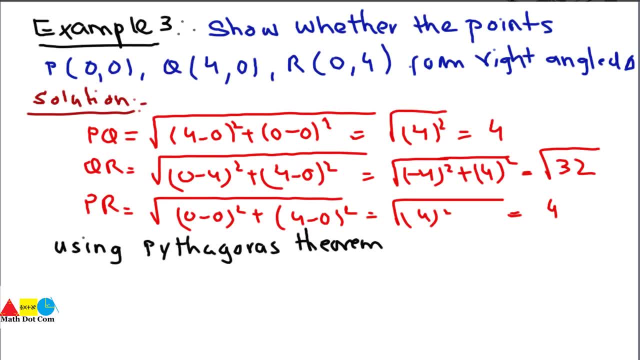 angle triangle. So for applying the Pythagoras theorem, first we will draw it on the graph so that we can easily understand which one is the hypotenuse, which one is the base and which is the perpendicular. So let us draw it on the coordinate plane. Here we have a coordinate. 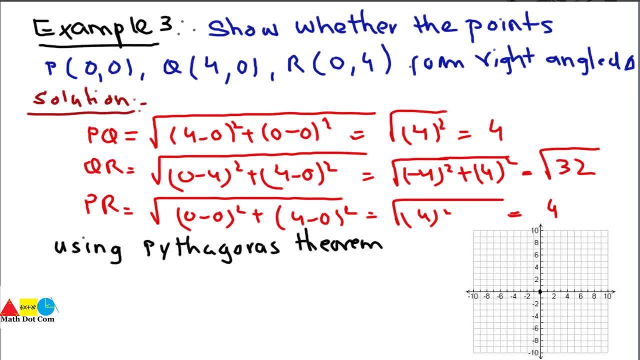 plane. So let us plot the points on the plane as first we have point P00.. This is P00, as this is the origin P00.. Then we have Q40.. It means here y is 0 and x is 4.. It means this point lies on. 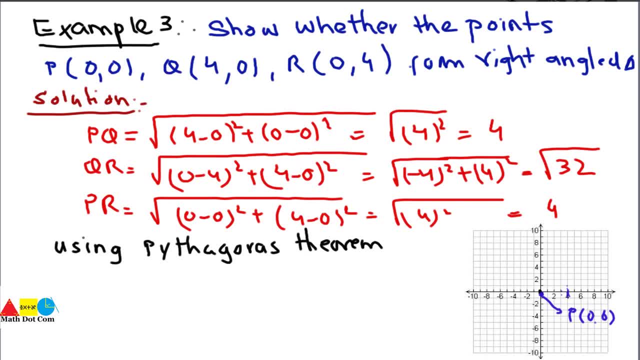 x axis. This point is the point Q, that is 40. This is the Q point, And then we have R04.. This is r. that is 0, 4. okay, so this is how we have plotted the points, and join them together to: 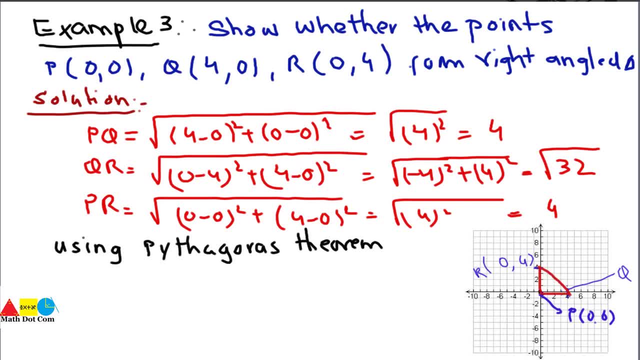 point to form a triangle as like this. so this is a triangle. okay, so it is clear from the graph that it's a right angle triangle. so we can also prove using Pythagoras theorem, as it is clear from here. the hypotenuse here is r, q, or you can say q r, so we can write as: q r square is equals. 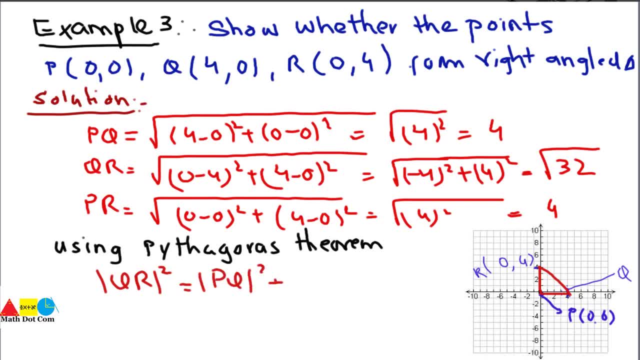 to base is p? q square plus perpendicular is p r square. okay, so q? r is what that is under root. 32 it's a square and p? q is what it's 4 square plus what is p? r? that is also force, okay, it's. If we cancel this, we will get: 32 is equals to 4, square is 16 plus 16 and 32 is equals to 32.. 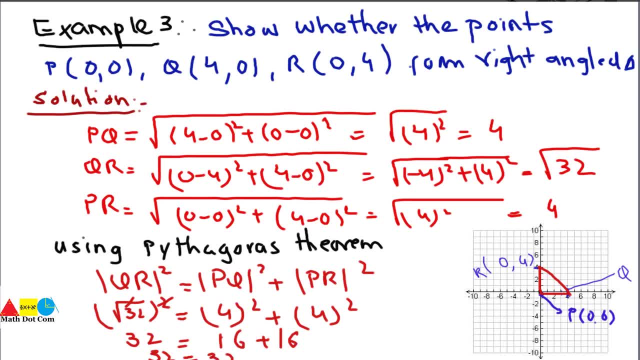 So it is clear from here that this is a right angle triangle, as, using the Pythagoras theorem, we have proved that the hypotenuse square is equals to the base square plus the perpendicular square. So this is how we can show that the given coordinates belongs to a right angle triangle. 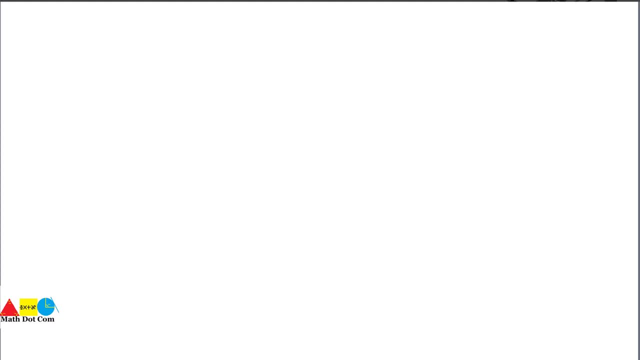 Let us have one more example to check whether the coordinates form a scaling triangle or not. So the example number 4 is: show that the point P, 1, 2, Q, 2, 1, Q is minus 2, 1 and R is 2: 1 forms a scaling triangle. 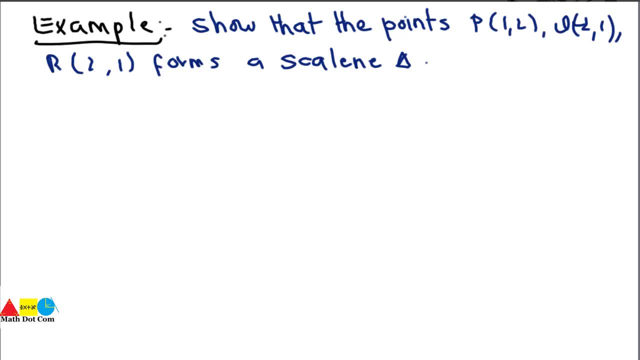 So we have already seen about the at the way start, about the scaling triangle. It is a triangle having All the sides different, So let us use the distance formula in order to find the sides of a, in order to find whether the sides are equal or are of different length. 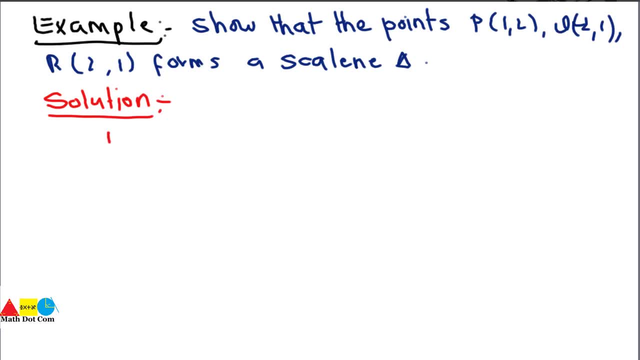 So first we will find P Q as X 2 is minus 2 minus 1 whole square. plus 1 minus 2 whole square, That will be equal to minus 3 square plus minus 1 square. Now it will give us, with the under root, 10.. 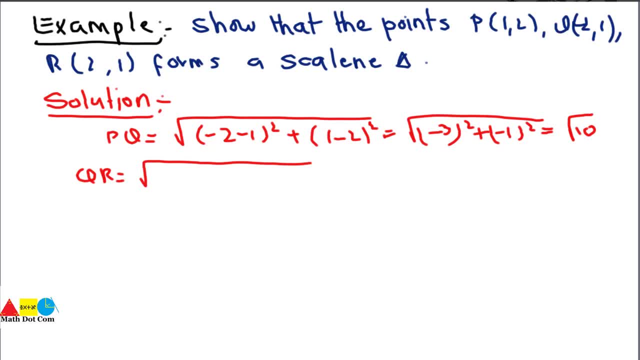 Then we have Q R. that is equal to Q. R is X, 2 is 2 plus 2 whole square. plus Y 2 is 1 minus 1 whole square. We will get under root 4 whole square. that is equals to 4.. 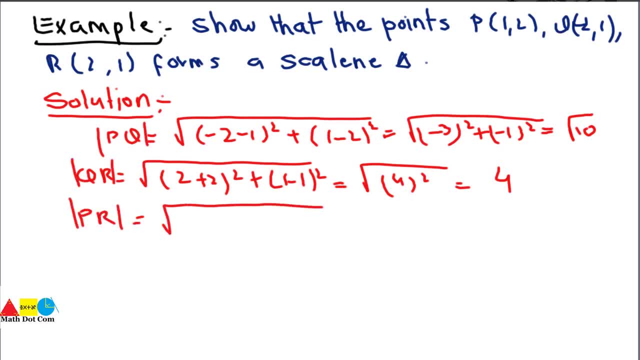 Then we have P? R. P R is equals to: we have X, 2 minus 1.. 1 whole square plus 1 minus 2 whole square will get 1 plus minus 1 square. It will be 1 and we will get under root 2.. 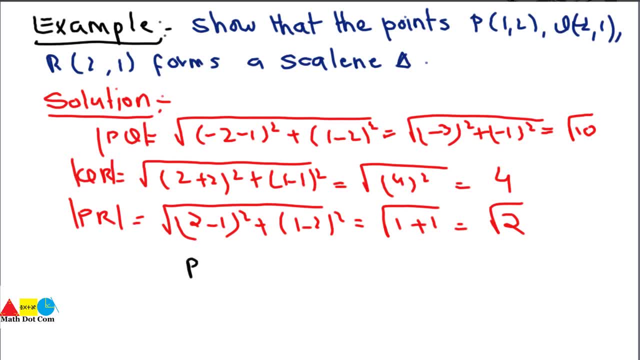 So it is clear from here that all the sides- P Q is not equal to Q, R is not equal to P R. Okay, So this is how we can say that the given points forms a scaling triangle. So I can write as given. 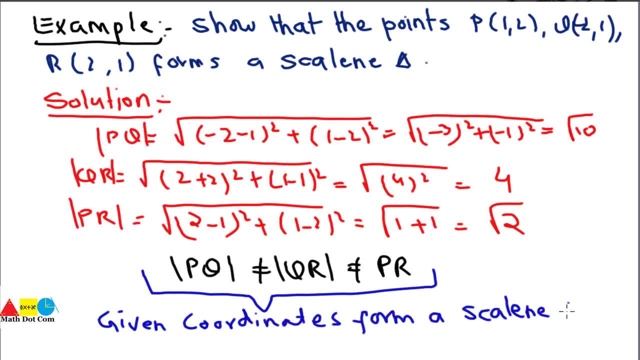 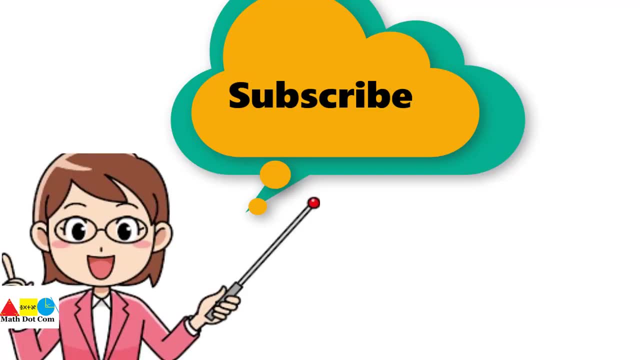 Given coordinates form a scaling triangle. So this is how we can check whether the given coordinates form which type of triangle: Whether a scaling or right angle, or isosceles or equilateral triangle. Thank you, Thank you for watching. If you like this video, please don't forget to subscribe our channel, mathcom, for more updates. Thank you, Thank you.